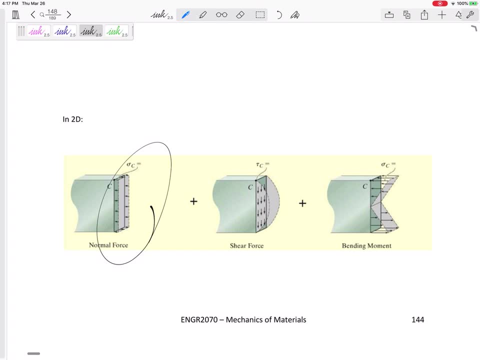 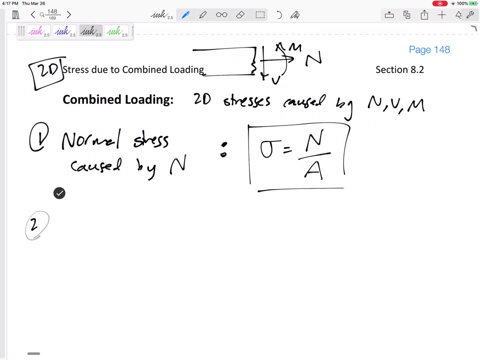 stress. so it is perpendicular to the cut and that would be compression right here of N over A, N over A, just the force divided by the cross-sectional area. all right, Let's look at V. V creates a shear stress. 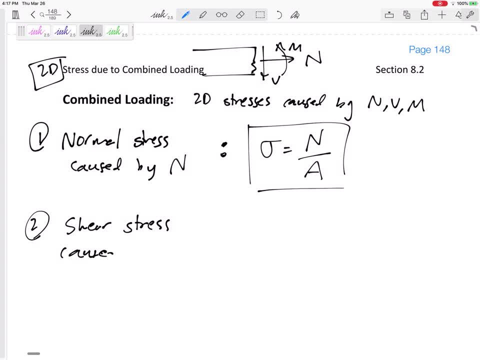 so let's look at the shear stress caused by V. Now we've already done this. Our old method, our old way was: tau is V over A. That's what we were using when we were designing pins. That's what we were using when we wanted a really quick 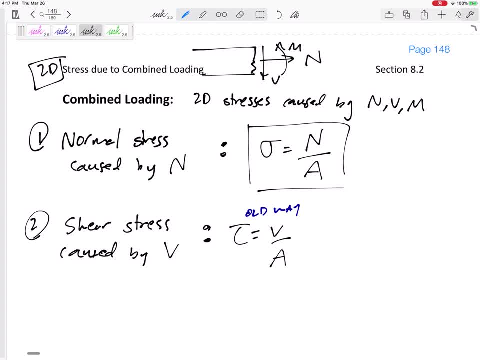 a way of figuring out what's the order of magnitude, what's the stress. we would find the tau average was V over A. But our new way, and our more accurate way is VQ over IT, VQ over IT. So now, 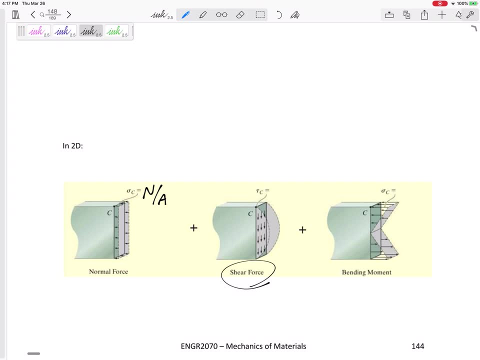 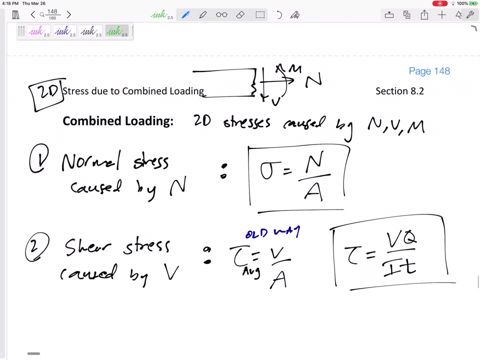 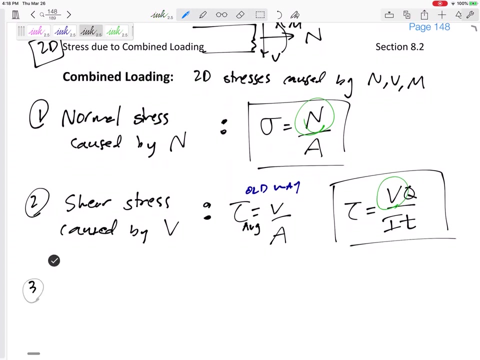 the shear stress caused by the shear force is VQ over IT. So you know, the N creates that stress, the V creates that stress. And what stress does the M create? This is what we've done. the bending stress caused by M- And it was sigma- equals MY over I. The book's going to say negative MY. 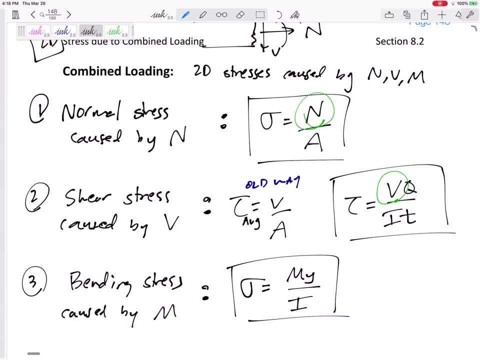 over I. I like to say MY over I and I'll give it a negative or positive myself after I look whether it creates a smiley face or a frown, and whether I'm looking at the top or the bottom. But this is, sigma equals MY over I. 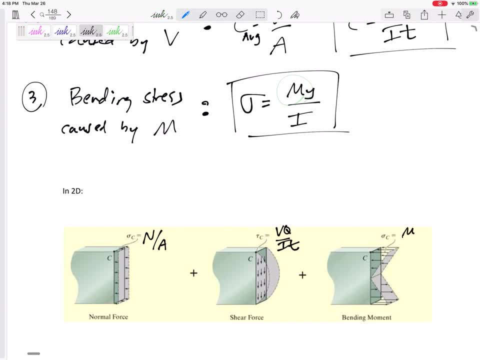 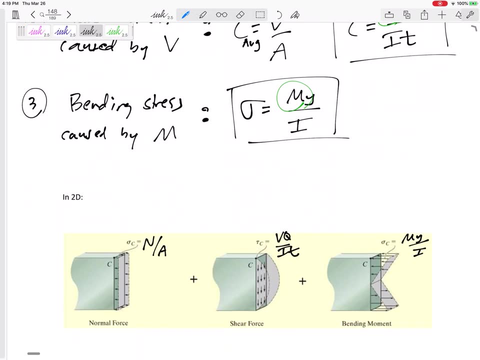 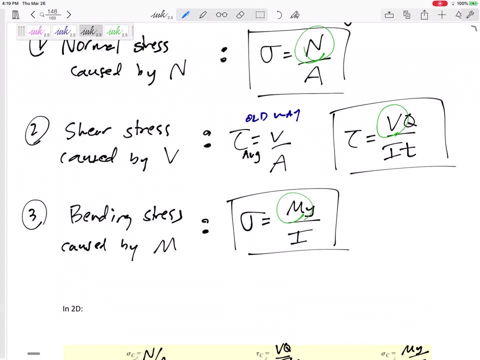 So that M creates this sigma. This would be MY over I. And do you see that both of these are sigmas? Both of these are perpendicular to the cut. They're compression or tension. They create elongation or contraction. This is a normal stress caused by M.